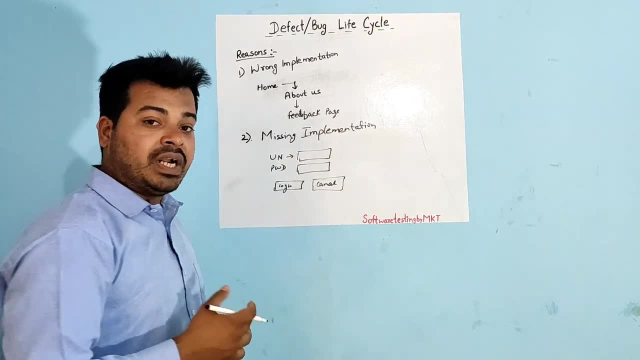 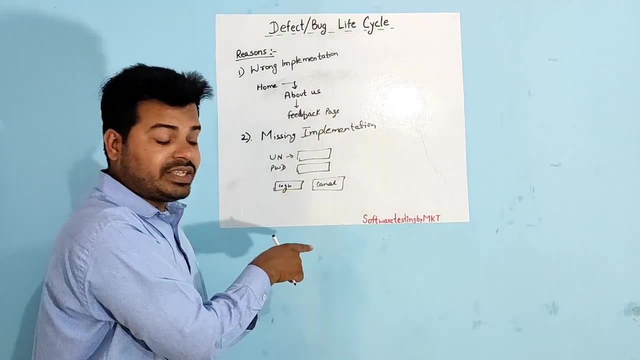 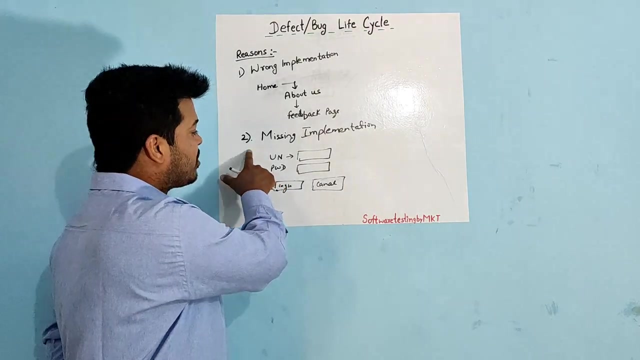 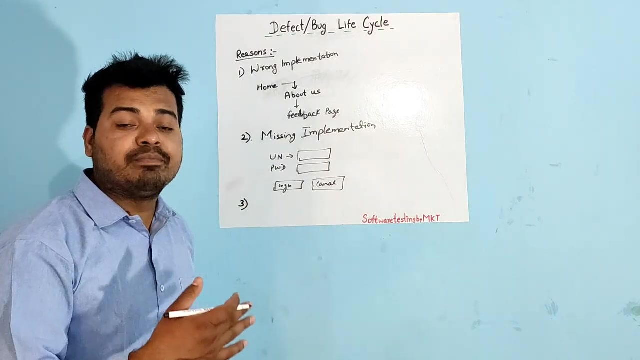 be cancel button. but when I have developed the software I have forgot to add this button. so missing implementation. you have missed this button to implement it in your software. so we will say it is a defect. it is called as missing implementation. now the third reason we get defect is called as extra implementation. suppose my requirement says that in my login. 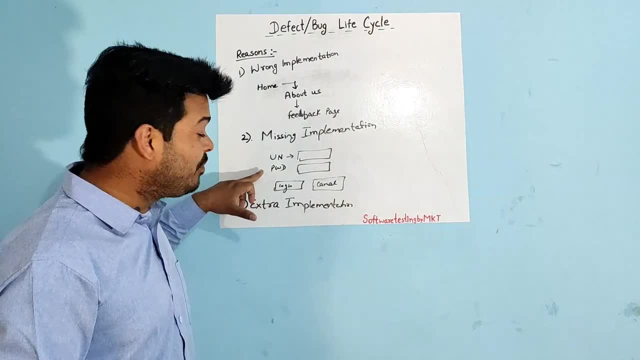 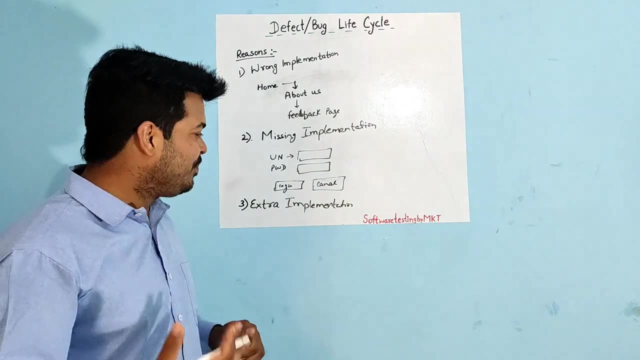 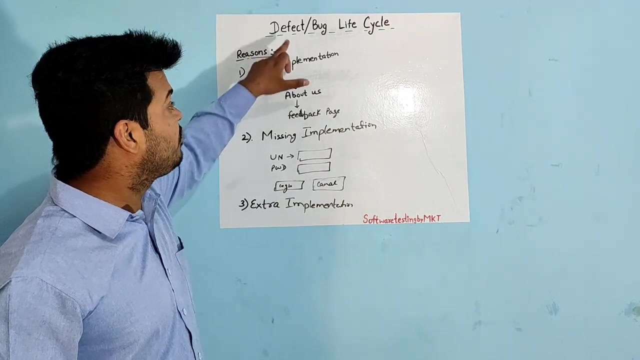 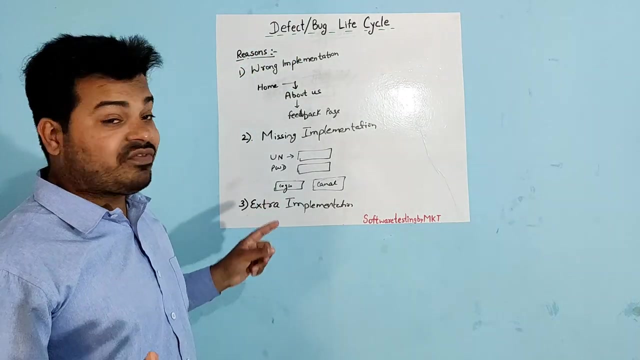 page. there should be user name button, there should be password button and there should be login button. that's all. but my developers when they were developing the software, they have even developed the cancel button. this is extra implementation which will be the reason of raising a defect by the text engineers. so these are the main reason why we raise. 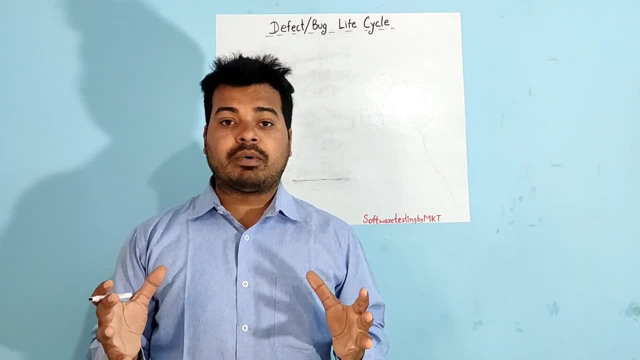 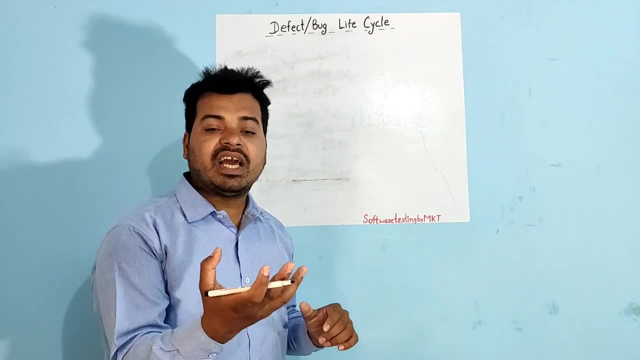 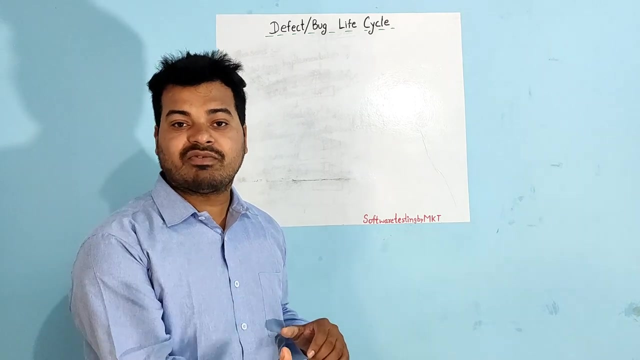 defect in the software. now we are going to talk about. what do you mean by defect in the life cycle in detail? so when text engineers, when they are raising any defect, when they are thinking the features or functionality it is not working according to the customers requirement, they will race the defect. so when they will raise the defect, the status of that. 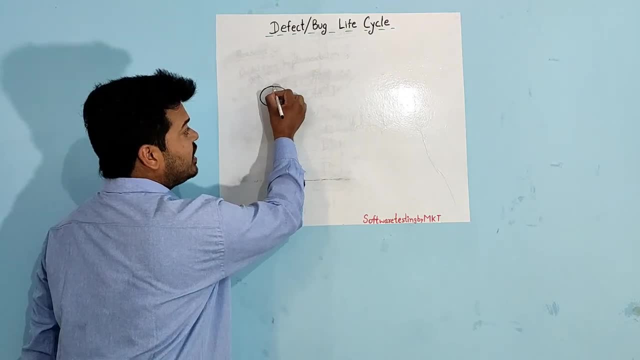 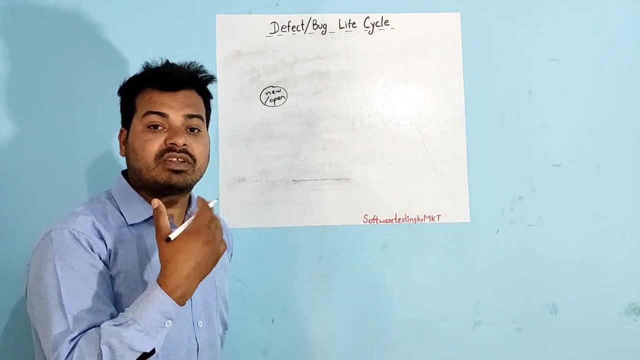 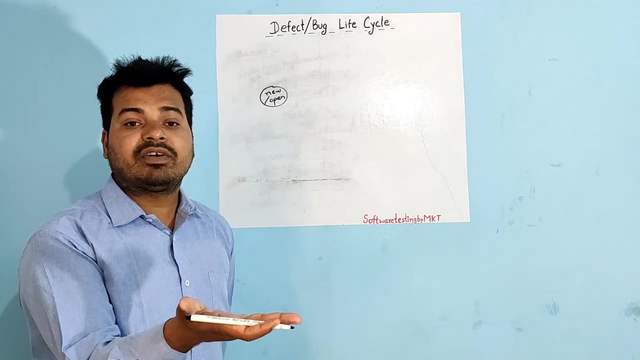 defect will be new or it will be open. they have raised it for the first time, that defect. since it was difficult, they have been given a code to get the defect to the user. so if that feature or functionality it was not working according to the customer's requirement, so they. 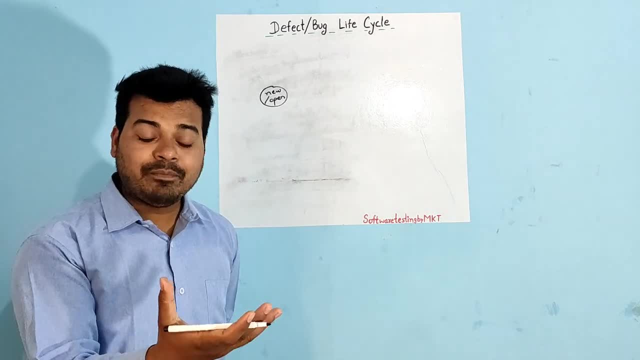 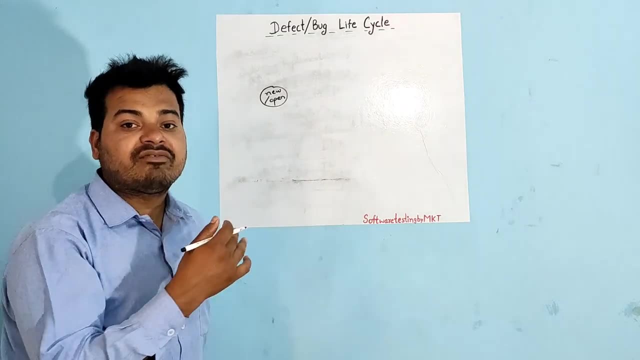 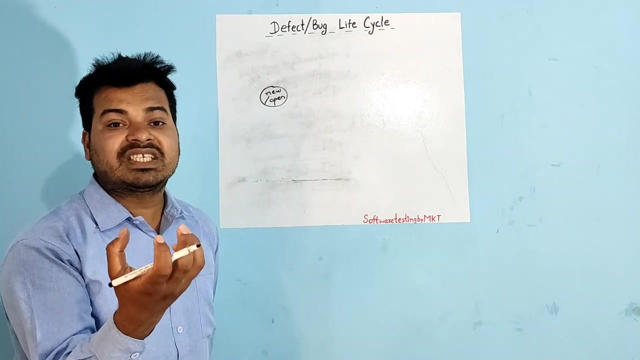 raised the defect. when they have raised it for the first time, the status of the defect will be either new or open. after raising the bug, they have to communicate with the development lead, whichever feature they were testing, if the test engineers know that this feature was developed by. 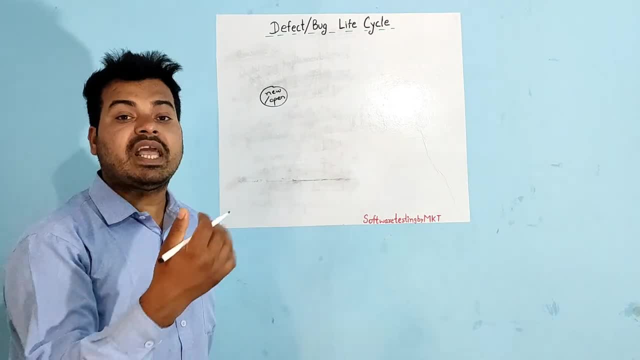 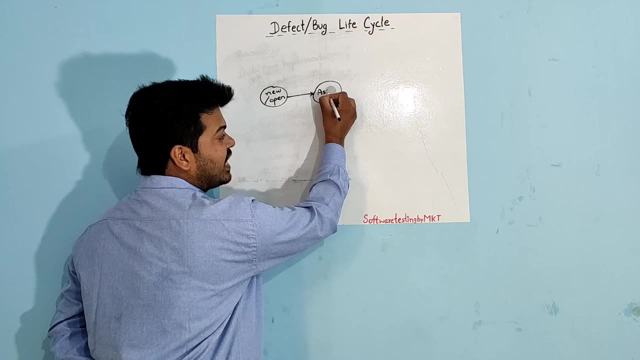 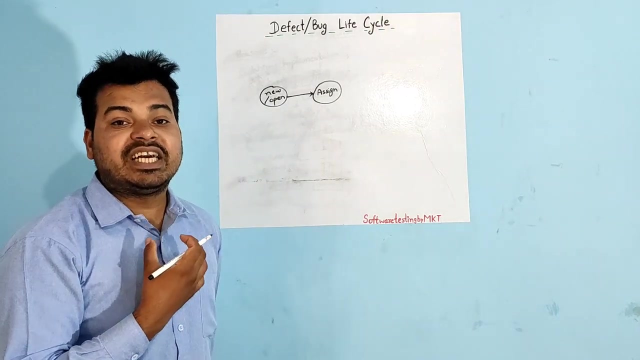 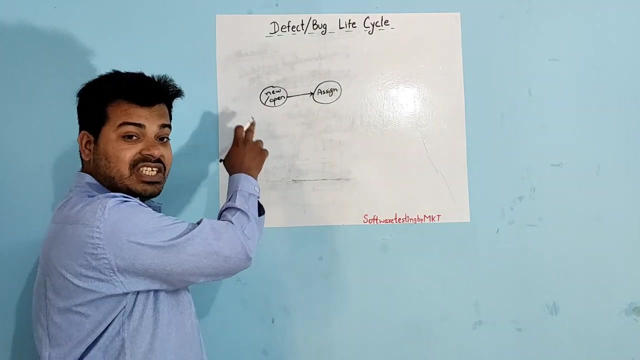 a particular developer. if they know, if test engineers know the name of the developer, they can easily assign it to the. they can easily assign to the respective developer. but if my test engineers they don't know this component or this module or this feature is developed by which developer, then test engineers will will communicate that bug with the development. 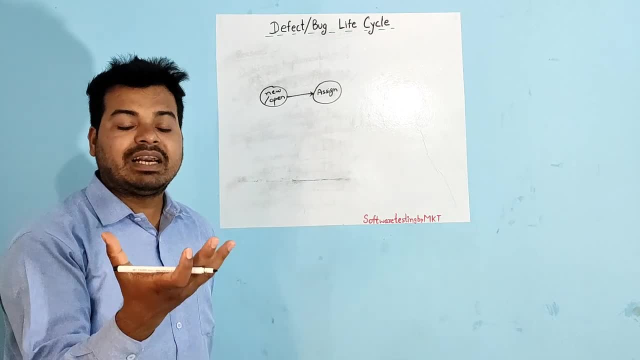 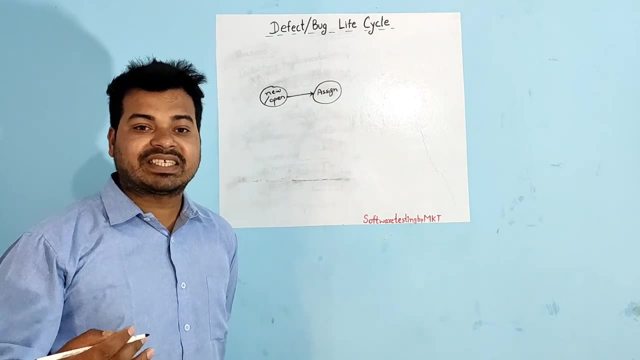 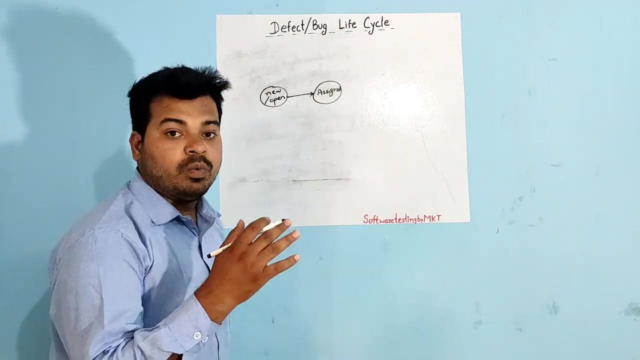 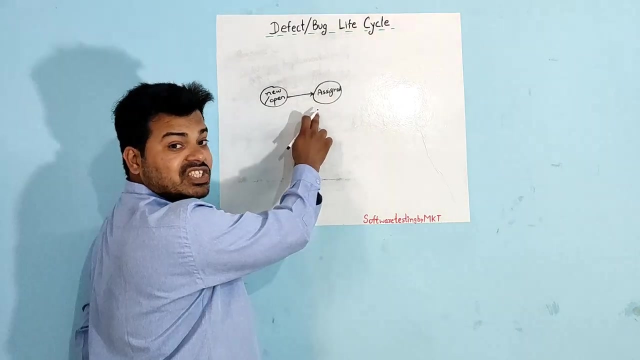 lead and finally, development lead will assign that particular defect to the respective developer when he's assigned. when development lead is assigning that defect to the new developer, the status of the defect will be assigned. once after developer has understood the bug and he has given the fix, he will change the status of the bug. 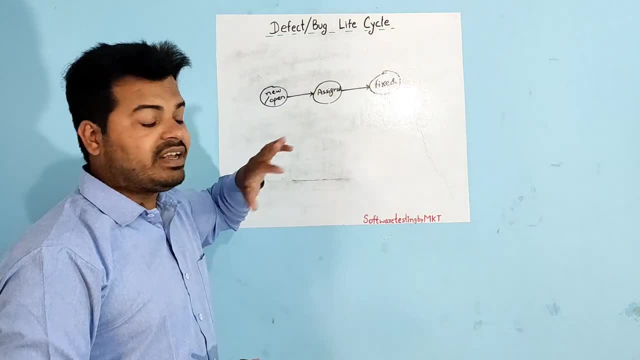 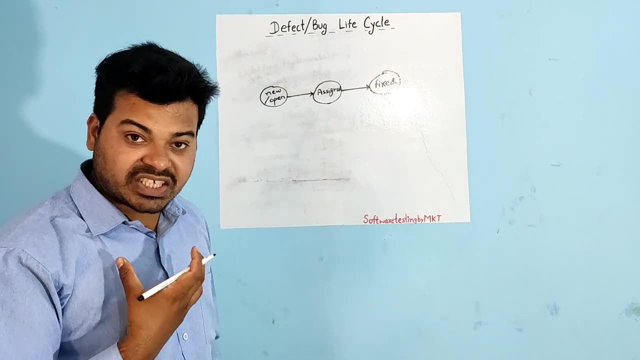 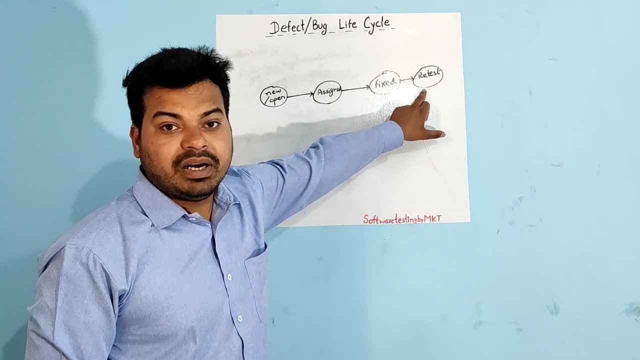 from assigned to fixed. here developer will change the status of the bug from assigned to fixed. now it is a responsibility for the test engineer to retest this fixed bug. retest it. retest is nothing but it is done by test engineers to make sure that, whatever the bug they had raised. 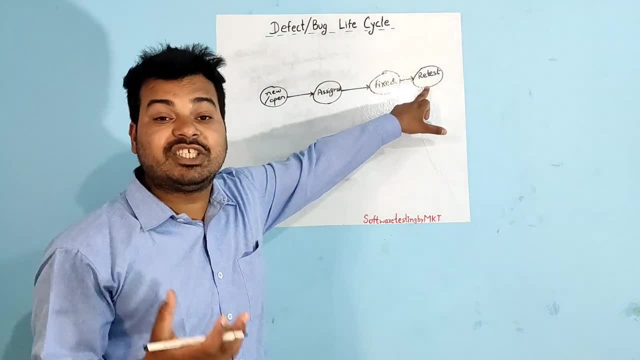 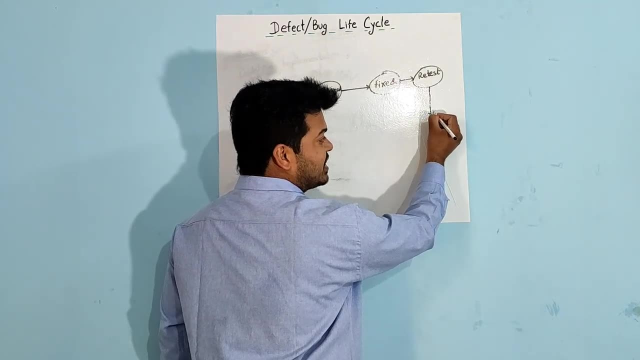 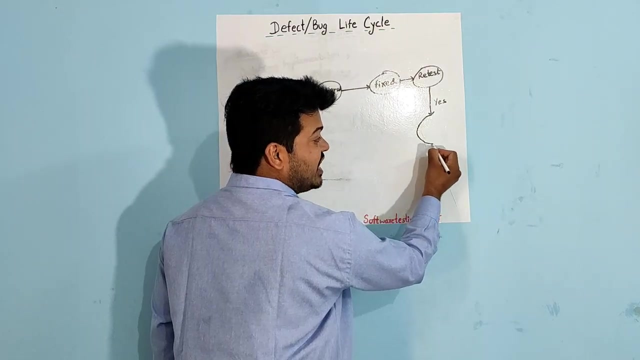 and it is fixed by the developer. now i am retesting it to ensuring that, whether it is really fixed or not, if, when test engineers are testing it, if it is really fixed, If it is really fixed, they will change the status of the bug. to close. 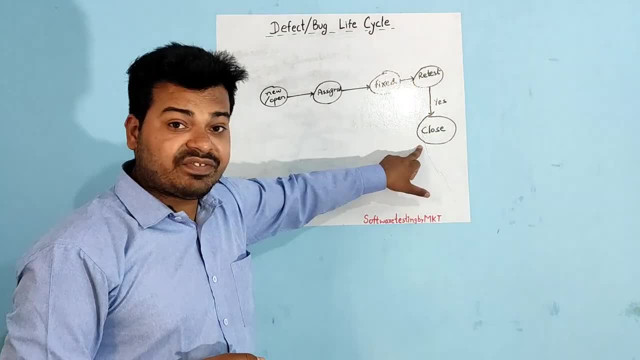 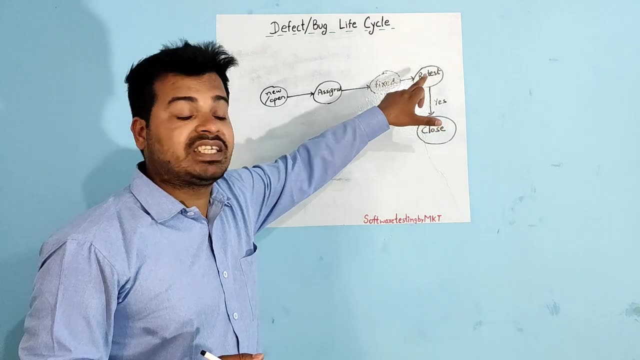 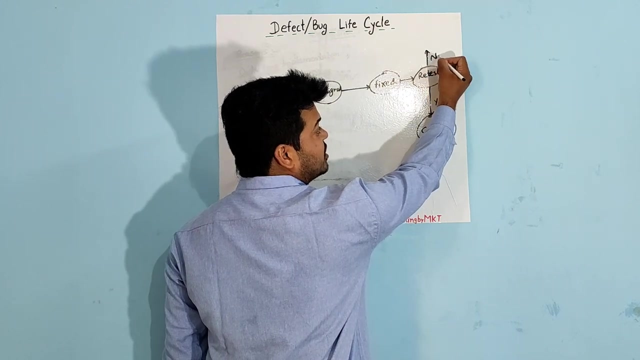 Test engineers when they are testing it. if it is really fixed then they will change the status of the bug from retest to close, Suppose, when test engineers are testing this defect, when they are doing retesting, and if that defect is not fixed, then they will change the status of the defect to reopen. Once after the status is changed to reopen, it will be assigned again to the particular developer. Developer will again give the fix. Test engineer will again do the retesting. If it is fixed, he will close it. If it is not, he will reopen it. So this is your bug life cycle. Other than that, there are multiple states. Suppose, when test engineers have raised any new bug and developers are not able to reproduce it, they can change the status of the bug to not reproducible. 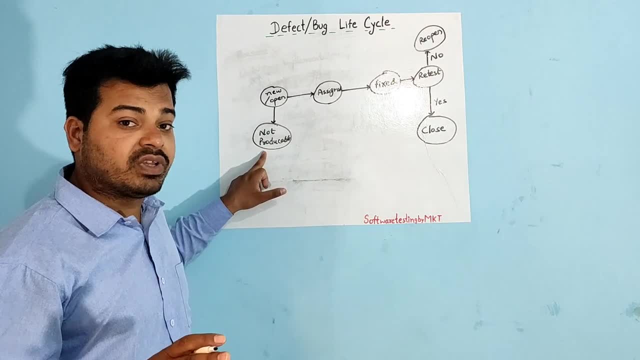 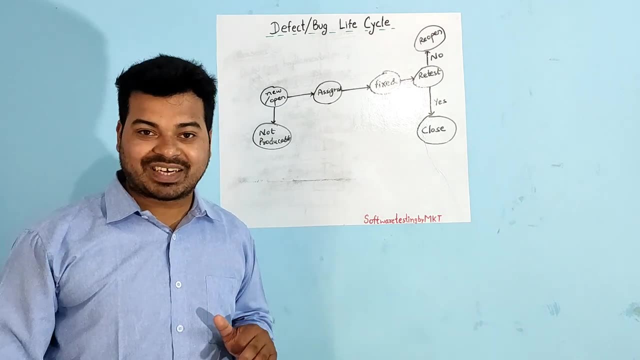 Developers can change the status of the bug to not reproducible if the steps to reproduce. Whenever you are raising any bug, you need to write all the steps to reproduce the particular defect. But when developers are not able to reproduce the defect, they can change the status of the bug. to not reproducible. not reproducible, There are other state also which is called as deferred defect. Deferred defect means minor defect. If developer is changing the status of the defect to deferred defect, in the sense they are telling that it is a very minor feature, Even though it. 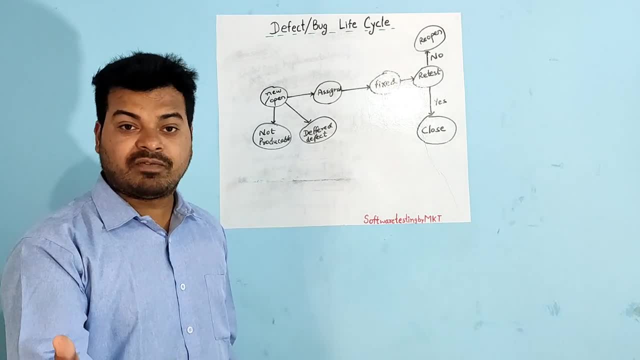 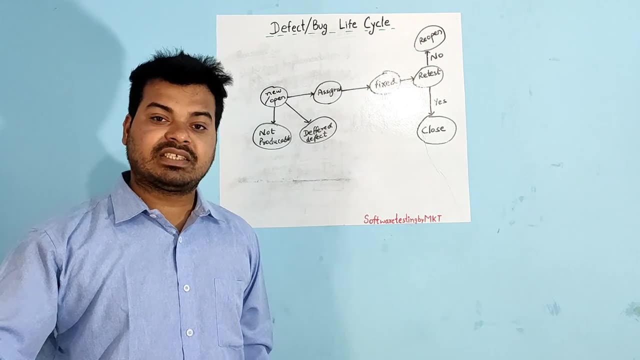 is not working. it will not impact my customer business workflow, But we are not telling that we will not fix it. We will fix it but in the upcoming releases. It is not going to affect the customer business workflow. So since it is a minor defect, we will fix. it in the later releases And there are other state also which is called as duplicate. The reason developer will change the status of the bug from new to duplicate is because whatever the bug they have raised is already raised by other test engineers or it is already raised.